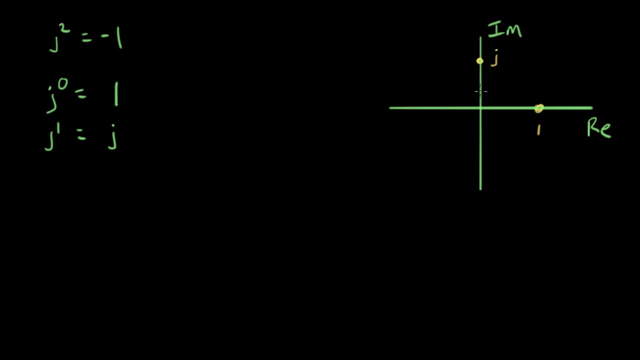 There's J. All right, this has no real part, It's all imaginary. Okay, let's keep going. Let's do J squared. And what is that equal to? Well, I wrote it down up here: J squared is equal to minus one. 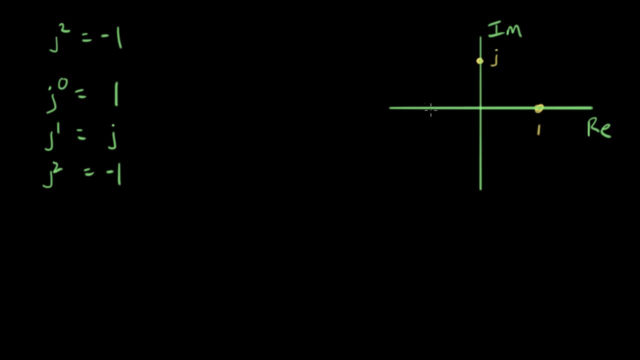 So J squared is equal to minus one. Where's that in the complex plane That's over here? at minus one On the real axis, no imaginary part. Let's do the next one. Let's do J cubed. What is that equal to? 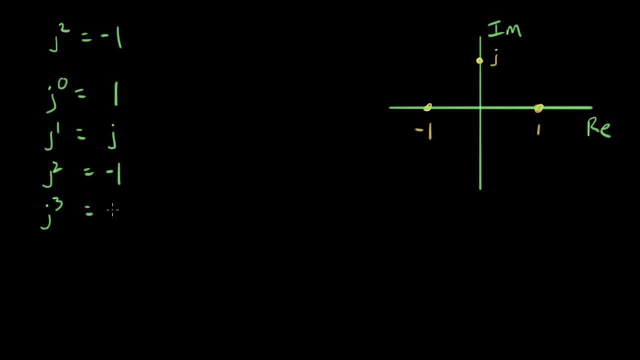 J to the third power is equal to- let's do J squared times J. And we have those two right here: J squared is minus one And J to the one is J, So that equals minus J. And where do we plot that? 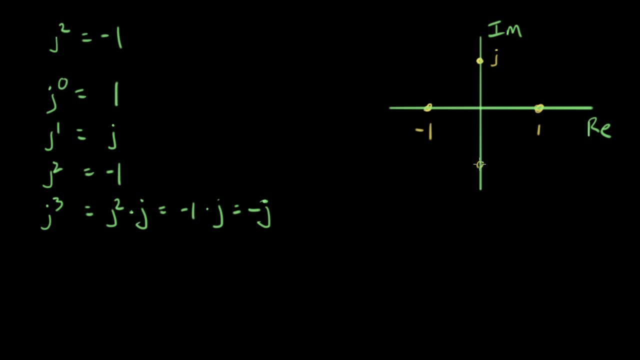 We plot that down on the imaginary axis in the complex plane right here, Minus J. Okay, now we've got four answers. Let's do one or two more. J to the fourth is equal to what? It's equal to J squared times J squared. 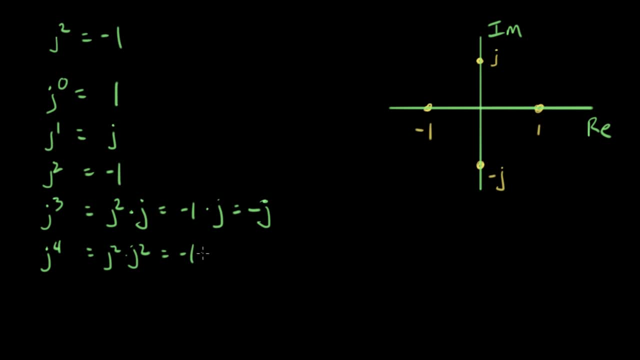 Let's look that up. It's minus one times minus one. And what is that? equal to That equals one. So let's go plot that. Well, we've already plotted it. So that's this answer, right here. All right, so we already have that. 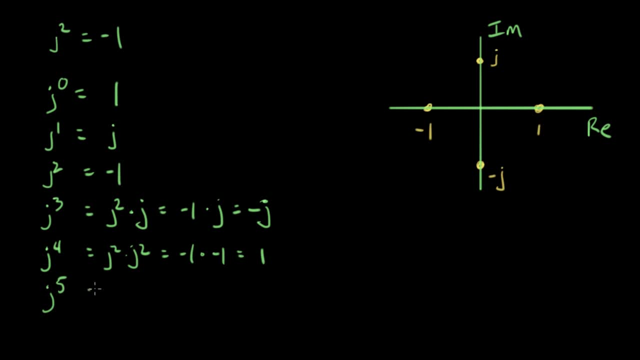 Let's do one more: J to the fifth. what is that equal to? That equals J to the fourth. That equals J to the fourth times J And J to the fourth is right here It's one times J equals J. Let's go plot that one. 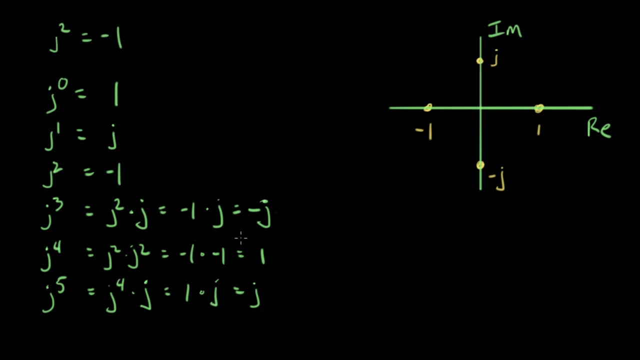 Well, we've already plotted it, It's already right here. Okay, so you can see there's a pattern here: One J minus one, minus J, One J, it's gonna be minus one and minus J. It keeps repeating, It keeps repeating. 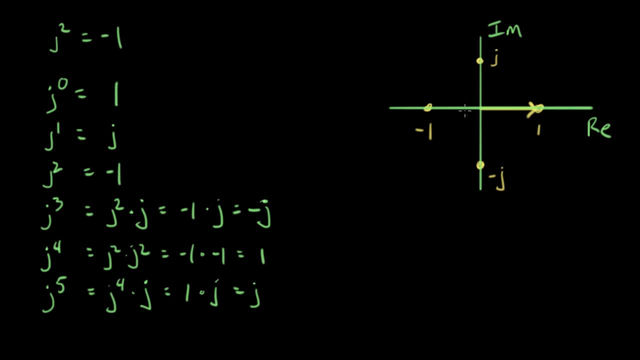 Here's what's interesting about this. okay, If we draw this as vectors, if I draw these imaginary numbers as vectors, when I multiply by J, when I multiply one by J, it rotated it 90 degrees. And then that was the first step, right here? 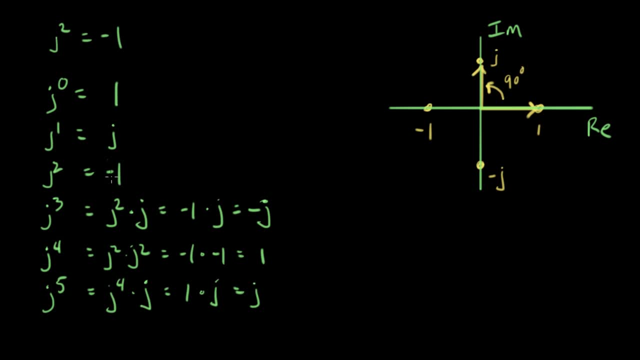 When I multiplied one times J, I got J. Now when we went to J squared, we ended up at minus one. So multiplying by J again caused the vector to go down here like that And that was another 90 degrees. And if I take it again, 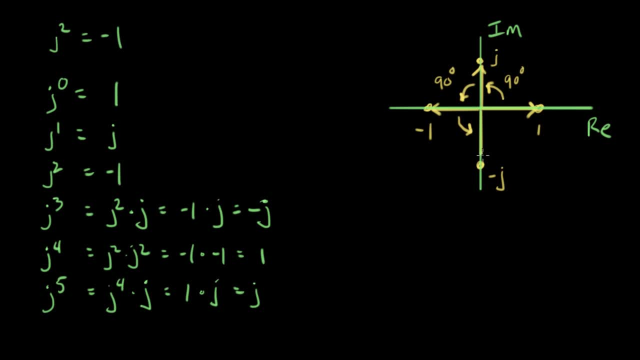 the next one went this way And the final one went this way. So this is the property of J. This is the key property of the imaginary unit. Multiplying by the imaginary unit, the nature of it is this: 90 degree rotation. 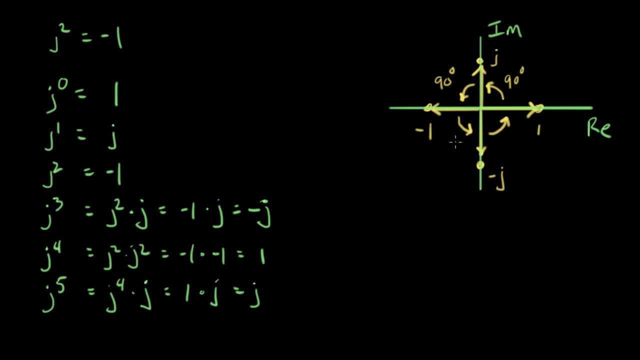 There's this idea of a number that causes other numbers to rotate, And that's the feature of J, that makes it super important And it's the reason that we use imaginary numbers in electrical engineering. So the key idea here is that J rotates. 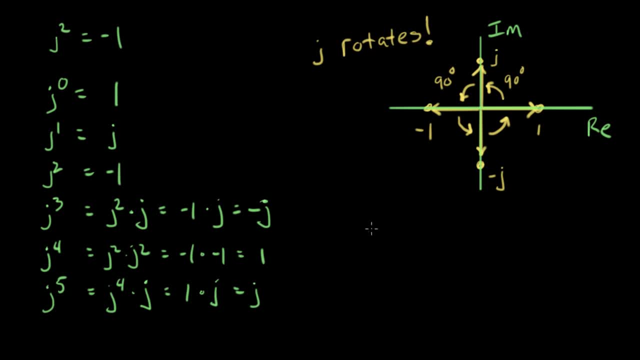 That's the point. That's what we love about J. So the last thing I want to mention is that negative powers, the powers of J. What happens if we have J to the minus one? Let's figure out what that means. So that, of course, is one over J. 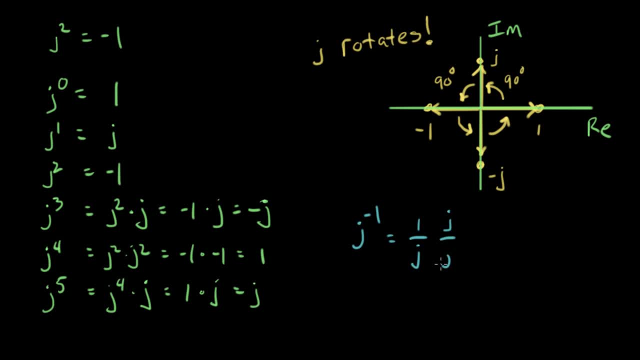 And if I multiply this by J over J and anything over itself is one, so I haven't changed the value of this- And that equals J on top over J, times J or J squared. And what is J squared equal to? We wrote it down right here. 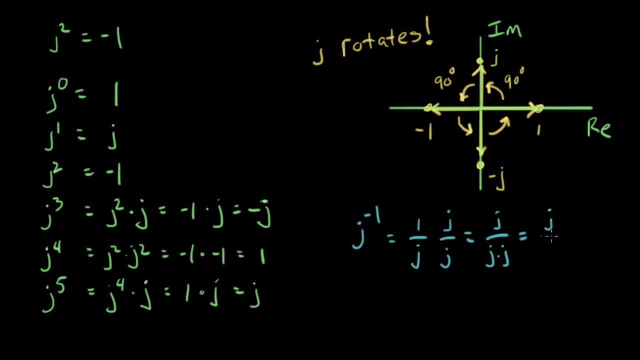 J squared is minus one. So this equals J over minus one or equals minus J. So whenever we see a J in a fraction, J to the minus one, basically it introduces a minus sign and the J comes up to the top out of the fraction. 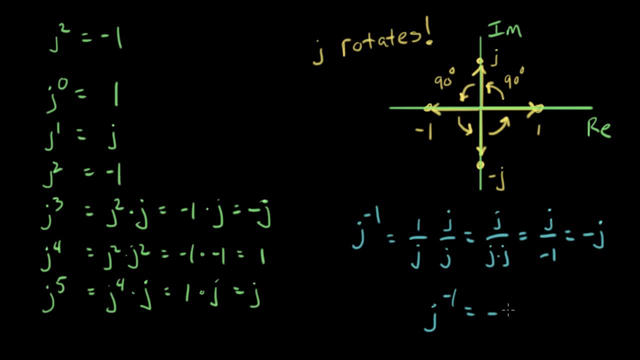 So J to the minus one equals minus J, And we'll use that occasionally to help us in our math. So this was a really quick review of complex numbers And if any of this was new to you, I really encourage you to go back. 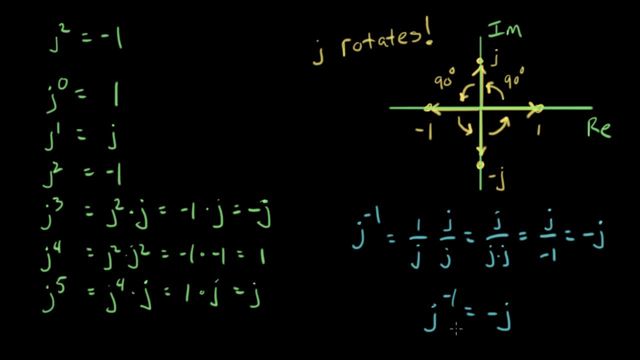 and watch Sal's videos on complex numbers, And if this is something you've seen before, I hope it knocked off some of the rust and we're ready to go and use these numbers.